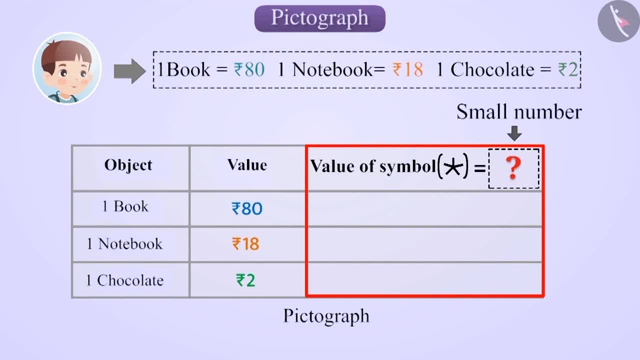 If you take the value of the symbol, a small number such as Rs 5,, then you will find it easier to denote Rs 2 and Rs 18.. But you will face difficulty while drawing many symbols to represent Rs 80.. 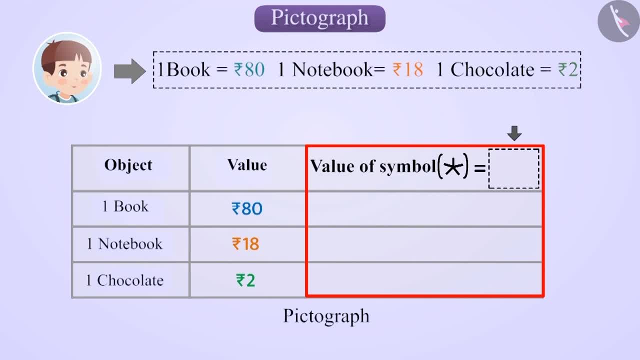 And if you take the value of the symbol, a larger number such as Rs 40,, then you will easily be able to represent Rs 80. But you will face difficulty while representing Rs 2 and Rs 18.. To overcome many such difficulties, we use bar graph. 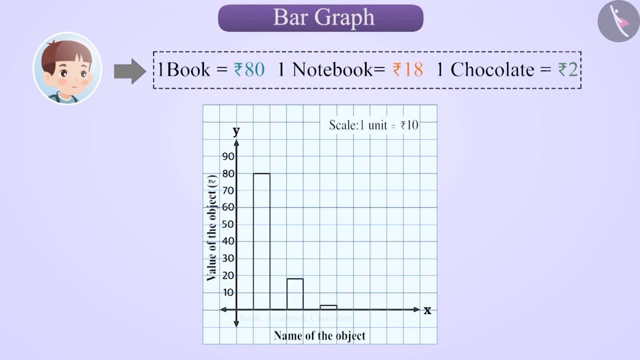 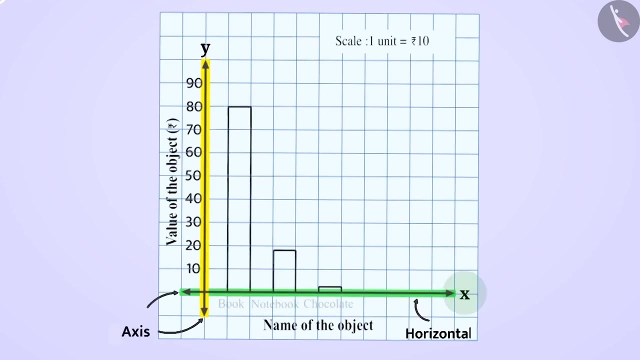 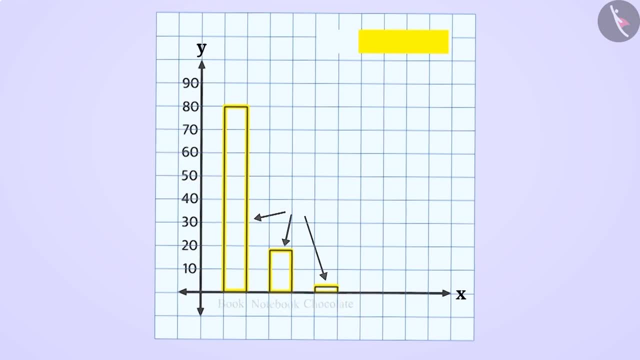 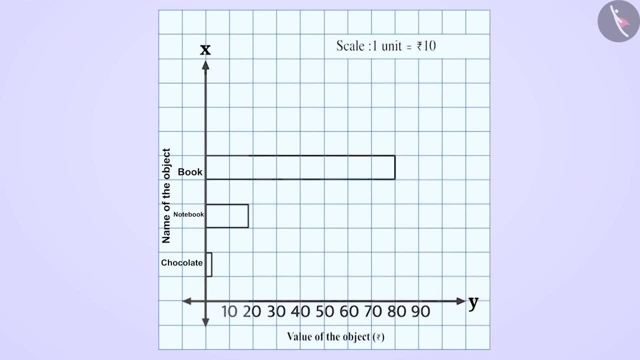 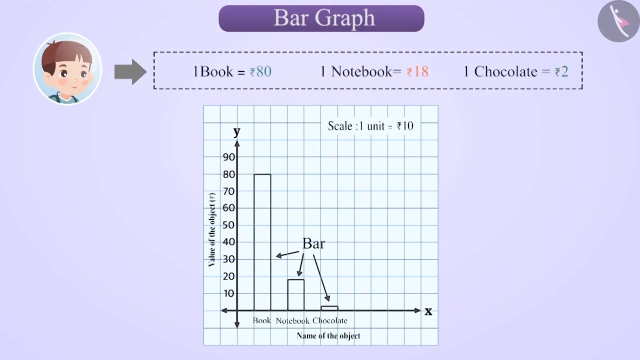 It is not necessary that the bar graph should be vertical. Instead, by interchanging the positions of the horizontal X-axis and the vertical Y-axis, we can also show the bar graph horizontally. The length of the bar represents the given number. Like here, we can say that the first bar denotes the value of the book as rupees 80.. 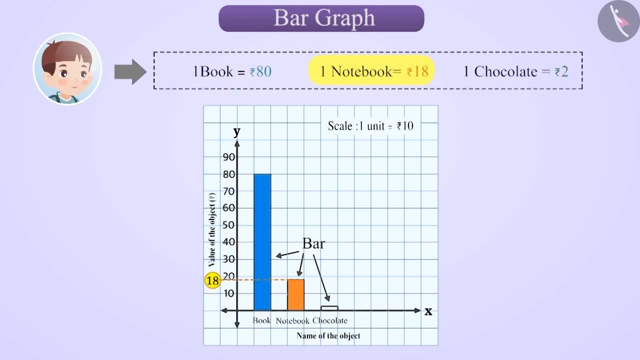 The second bar denotes the value of the notebook as Rs.18,, while the third bar denotes the value of the chocolate as Rs.2.. Thus we can say that the graphical method of representing the data where bars of uniform width are drawn horizontally or vertically 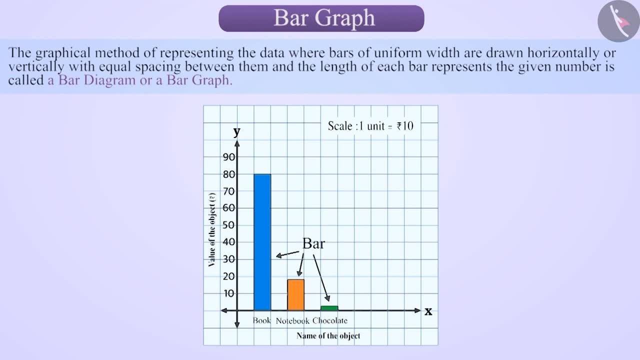 with equal spacing between them and the length of each bar represents the given number, is called a bar diagram or a bar graph. Just think what all information you can collect from a bar graph. Absolutely right. With the help of a bar graph, we can obtain different types of information. 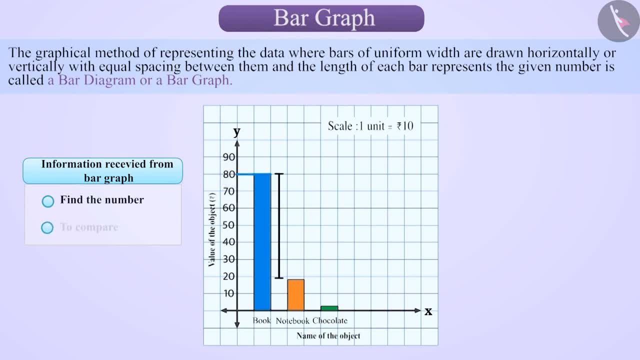 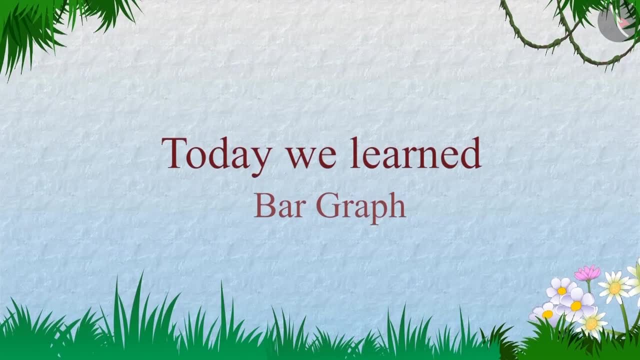 For instance, to find the number, to compare, etc. Today we learned about bar graph. In the next video we will learn how to draw a bar graph. Thanks for watching.